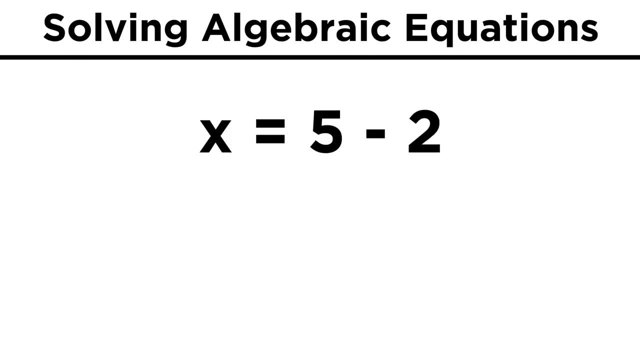 On the left, X plus two minus two leaves X all by itself, which was precisely the plan. On the right, we get five minus two, which is three, and therefore X equals three, the answer we were expecting. If we had something like N minus four equals seventeen, we'd have to subtract two from 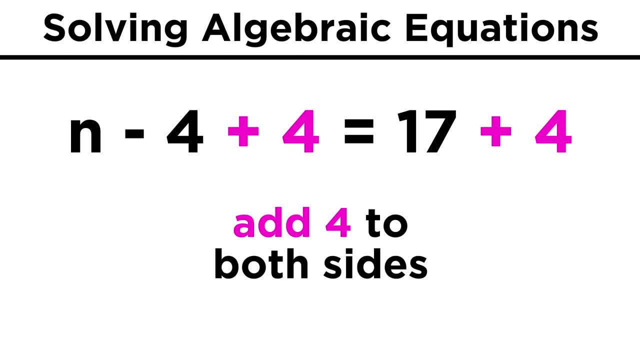 both sides, because addition is the inverse of subtraction. On the left we get N by itself. On the right we get twenty-one, so N is equal to twenty-one. This works the same way for multiplication and division. Given the equation four D equals twenty, we can see that the variable is being multiplied. 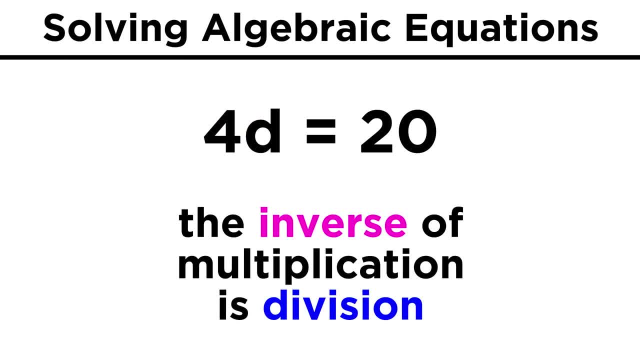 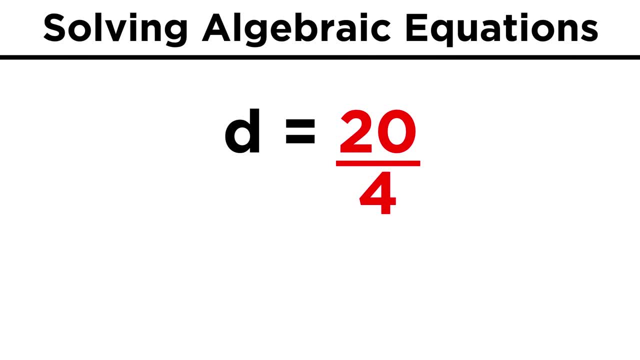 by four. The inverse of multiplication is division. so we have to divide both sides by four. On the left the fours cancel, and on the right, twenty divided by four is five. so D equals five, And if we have Y over eight equals three. we now have to multiply both sides by eight. 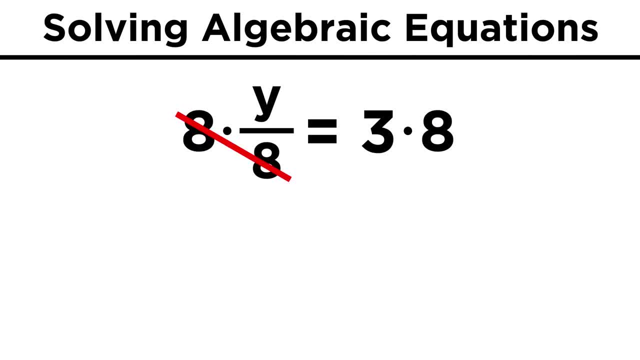 because the inverse of division is multiplication. On the left, the eights cancel, leaving us with Y, and on the right, three times eight is twenty-four, so Y equals twenty-four. How about something a little harder like: four minus B equals seven. 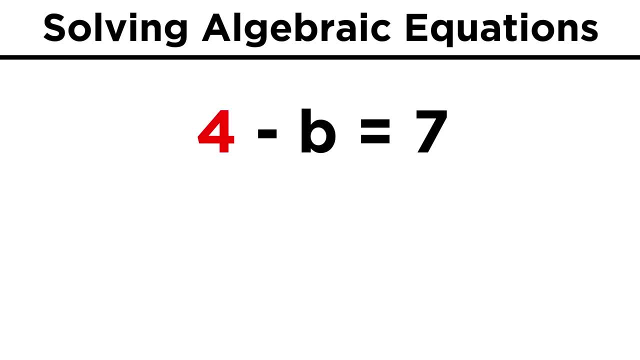 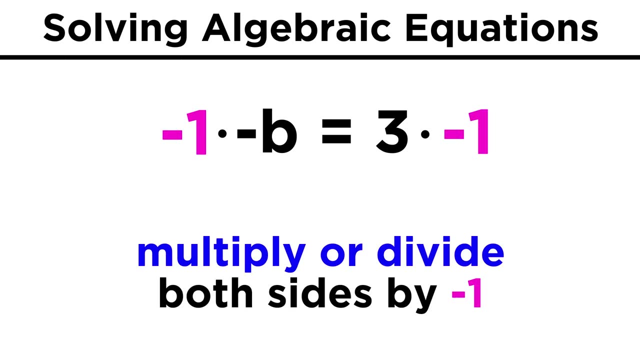 Order might look a little confusing, but we still just need to get rid of this four. so let's subtract four from both sides. That will leave negative B equals seven minus four, which is three. We want to know the value of positive B, so we just have to either multiply or divide. 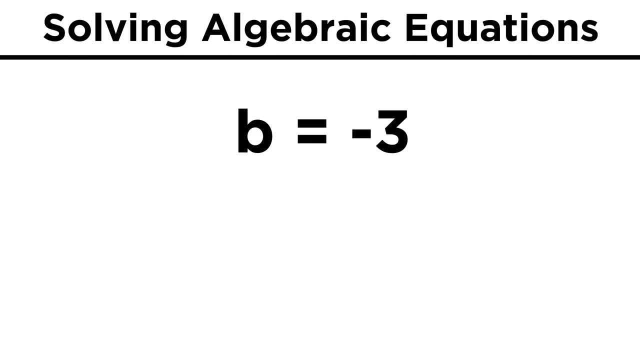 both sides by negative one. That will mean that B equals negative three. With this example, we can see that if we have two steps to do, we undo our first step, which is to divide both sides by negative one. We do operations in the reverse order of PEMDAS. 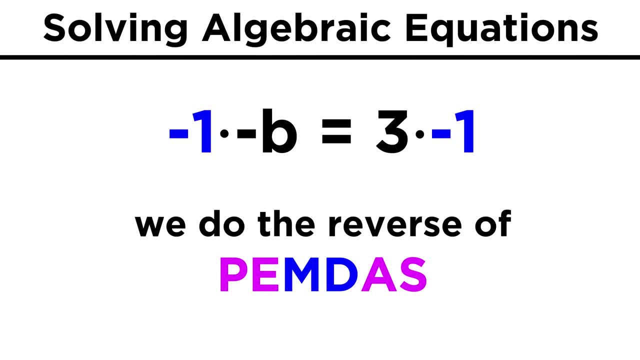 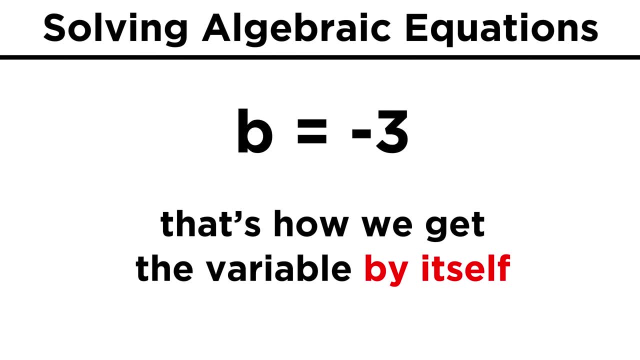 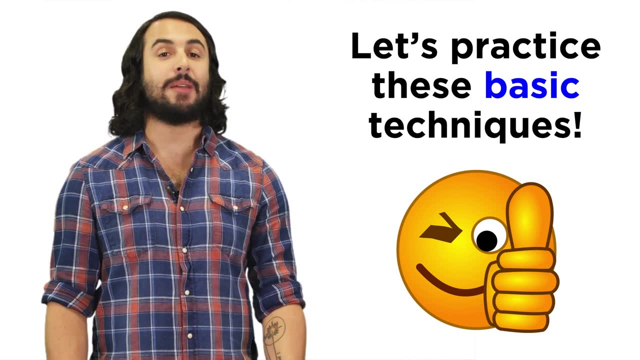 We work with addition and subtraction first, and then we do multiplication or division. This is the order that is necessary to get the variable by itself. Algebraic equations can certainly get much more complicated than this, but we should master these simple ones first. so let's check comprehension.